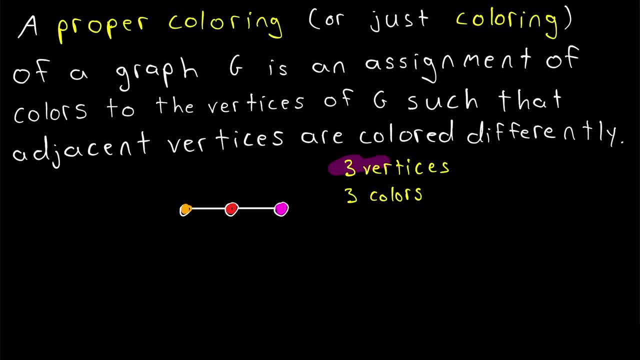 we've colored it with three colors. Certainly, any time a graph has n vertices, we'll be able to color it with n colors, Because if every vertex has a different color, like we have here, then certainly adjacent vertices will always have different colors. But when we talk about 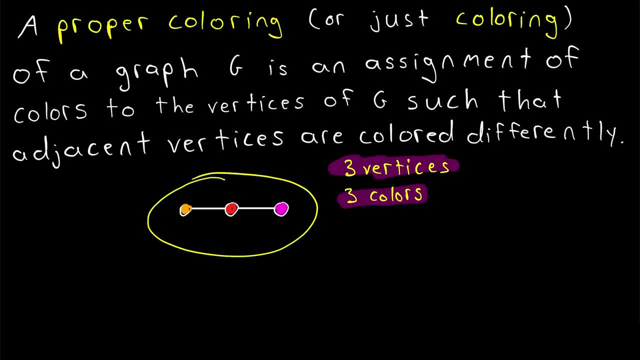 colorings. typically, our goal is to color a graph with as few colors as possible. In this case, is it possible that we could color the graph with fewer than three colors? In this case, it certainly is possible. This vertex here is adjacent to the orange one. 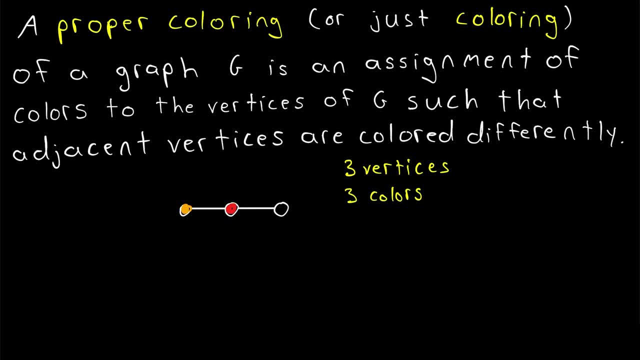 so it can't be orange. So we can color it red, just like we did before. This third vertex is adjacent to the red vertex, so it can't be red. However, there's nothing stopping this one from being orange as well, because it's not adjacent to the other orange vertex. 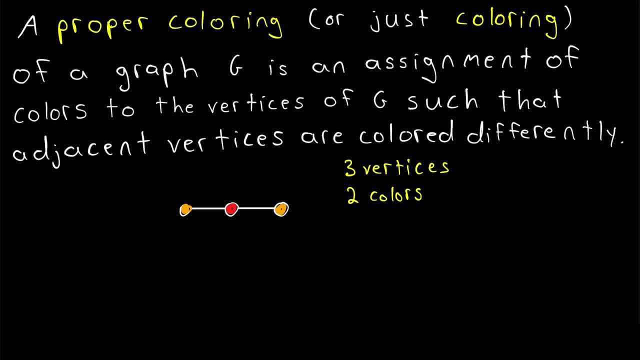 So now we've colored this graph that has three vertices with only two colors. And again, notice the important feature of how we've colored this graph: we've colored it so that adjacent vertices are colored differently. the red vertex has two neighbors and neither of them are red. Notice as well, since we 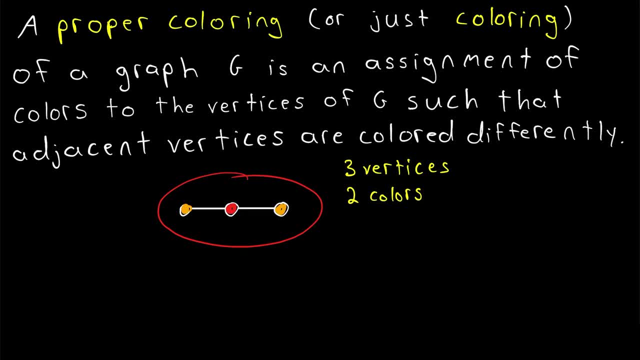 managed to color this graph with only two colors. that immediately tells us that it is a bipartite graph. we can put all the vertices of one color in one part tight set, and all the vertices of the other vertices will be colored in one color. This is a two color graph, which means that it 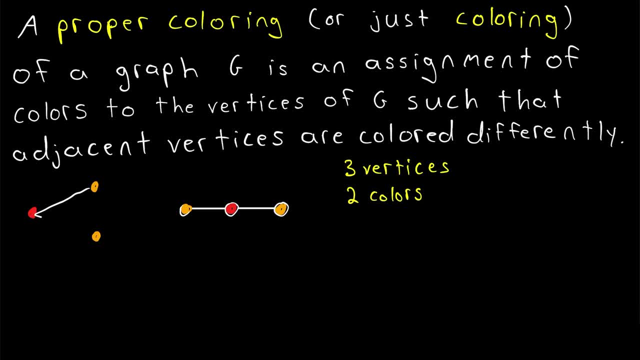 can be colored in any color. Notice how that's important In this case. the red vertex is other color in the other partite set. So clearly. coloring a graph with two colors demonstrates that it is a bipartite graph Vertices of the same color. by definition of a graph, coloring will not. 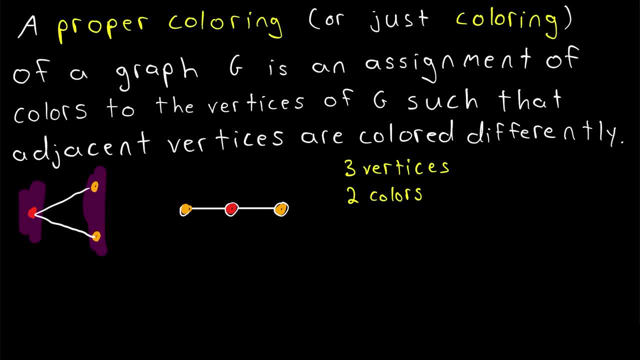 be adjacent so we can put them in their own partite sets. Notice, if we change our path graph into a cycle graph, it would no longer be bipartite and we also can't color it with just two colors anymore. Now our two orange vertices are adjacent, so we've got to change the color of one of them. 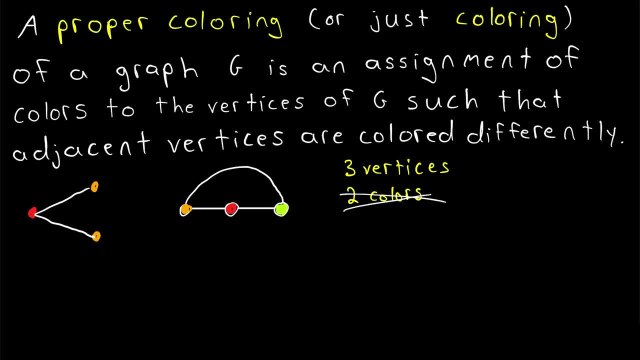 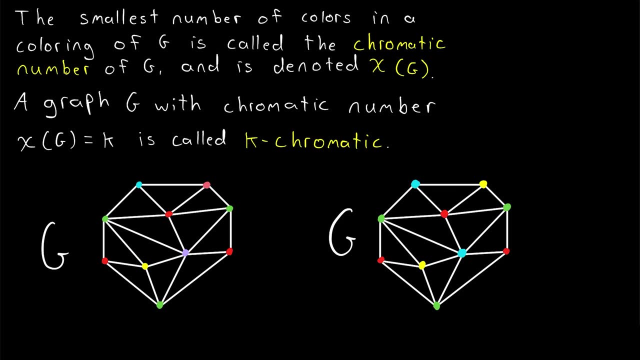 in order to keep a proper graph coloring. So one more time, a coloring of a graph g is an assignment of colors to the vertices of g, such that adjacent vertices are colored differently. All right, let's see some more of this language. regarding the coloring of vertices, Like we mentioned earlier, 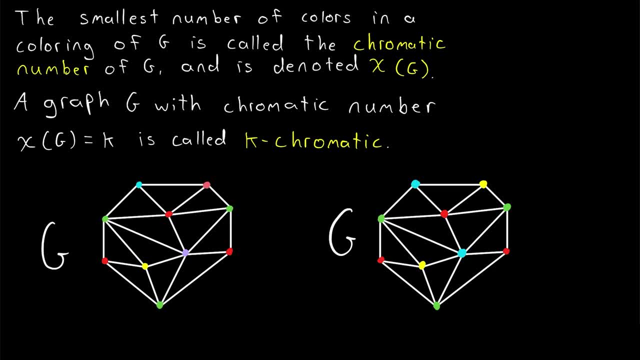 when we talk about colorings of a graph, we're typically interested in the color of the vertices of a graph. So we're going to talk about colorings of a graph. in coloring a graph with as few colors as possible- The smallest number of colors in a 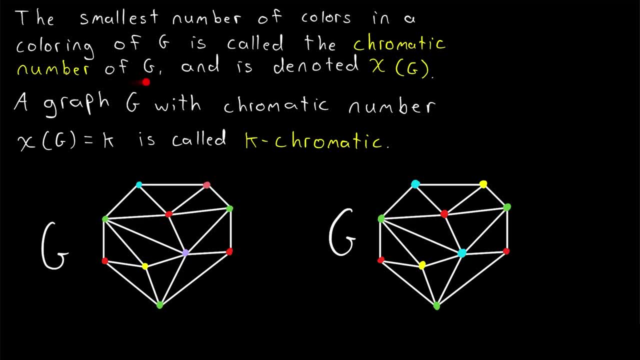 coloring of a graph g is called the chromatic number of g and is denoted like this: This is the greek letter chi of g, and a graph g with chromatic number equal to k is called k chromatic. So here's an example of a coloring of a graph g. Let me zoom in so that you can hopefully see. 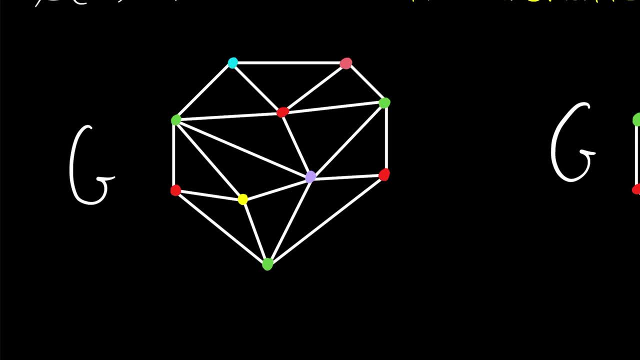 the colors a little better and notice that this is indeed a chromatic number of g. So this is a proper coloring of the graph. If we just look at a couple examples, consider this red vertex here. None of its neighbors are red as well. Look at another example. How about this? 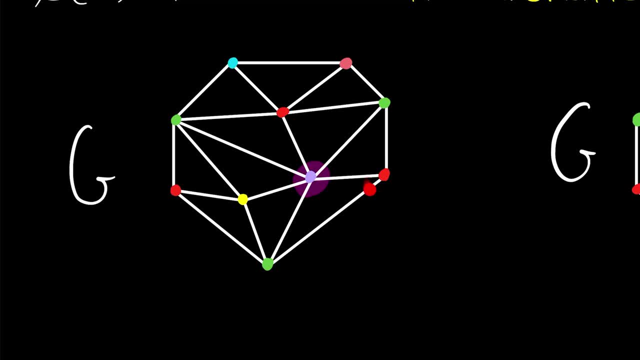 purple vertex. None of its neighbors are purple, So this is a proper coloring. you could confirm if you looked at every pair of adjacent vertices. No adjacent vertices will have the same color, So that's what makes it a coloring. Then we might ask how many colors are used here to color the graph g? 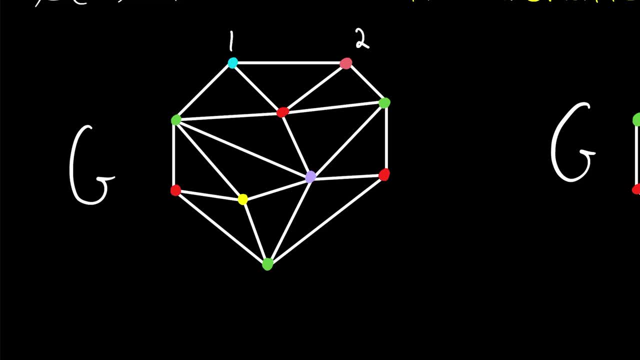 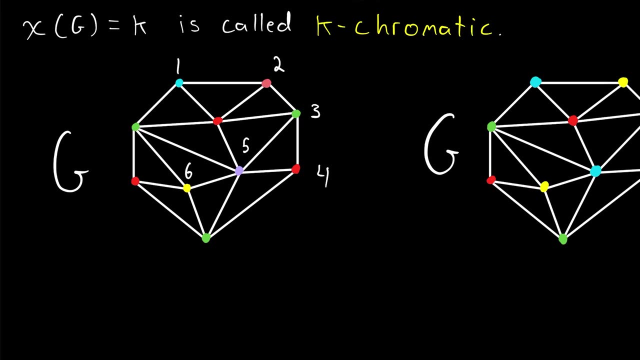 Well, if we count them up, looks like there's one color, two colors, three colors, four colors, five colors and then six colors, counting that yellow as well. So a total of six colors to color this graph. Is that the minimum number of colors possible? Well, we see, that is not by checking out. 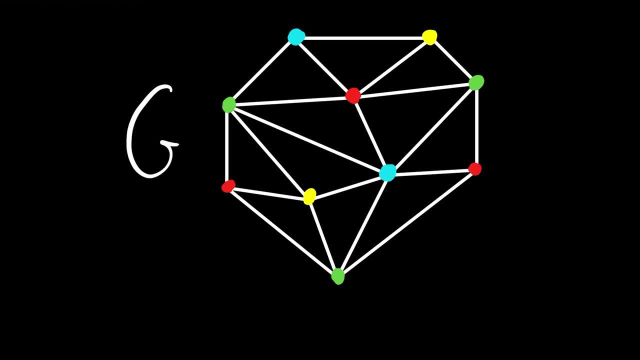 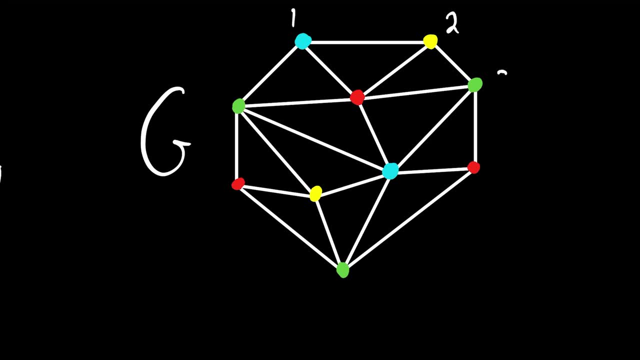 this other coloring of the same graph. This is indeed another proper coloring of the same graph. and how many colors does it use? Well, if we count them, there's one, two, three, four colors and it looks like that's it. We've only got blue, yellow, green and red used. 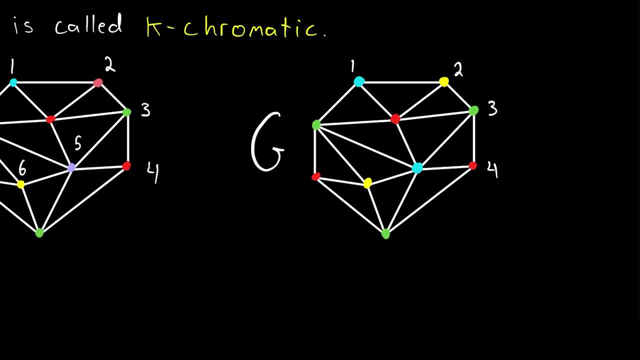 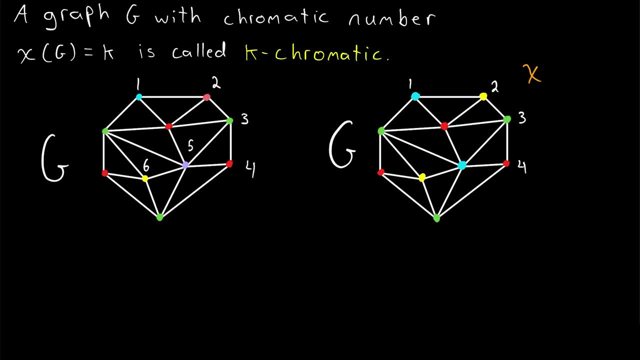 for the colors in this graph, And in fact four is the smallest number of colors we can possibly color this graph with. Thus, the chromatic number of this graph, chi of g, is equal to four. Again, that's the smallest number of colors in any coloring of the graph. So, since the chromatic 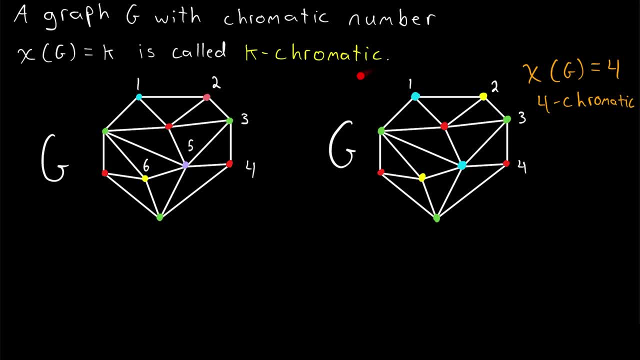 we could also say that g is four chromatic. If we tried to color this graph with, just say, three colors, then no matter how we went about doing it, if we only used three colors, some pair of adjacent vertices would have to have the same color. Again, we need a minimum of four colors in. 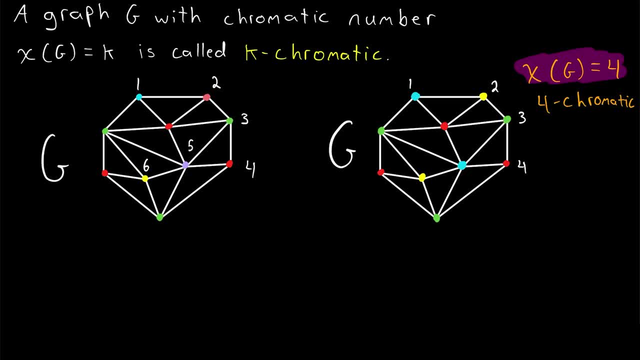 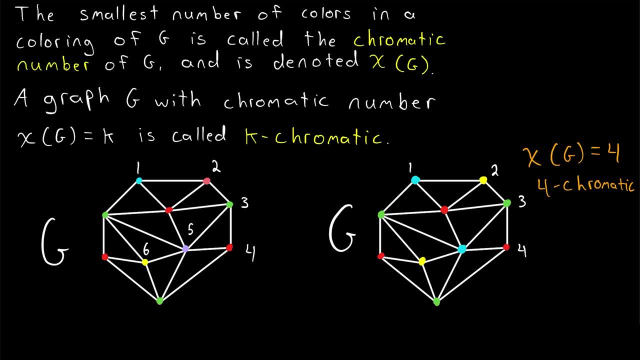 order to color this graph, and that's why it is four chromatic and has a chromatic number of four. All right, so one last time recapping that definition: The smallest number of colors in a graph, g, is called the chromatic number of g and is denoted chi of g, A graph with chromatic number. 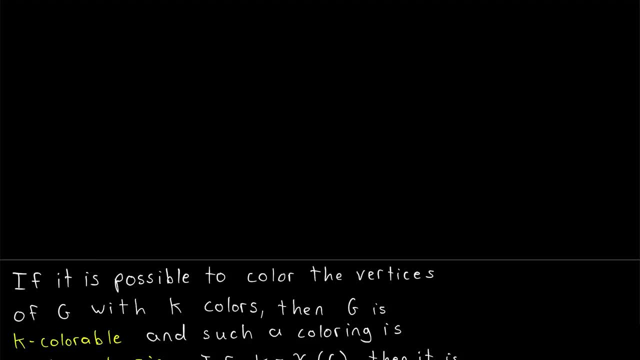 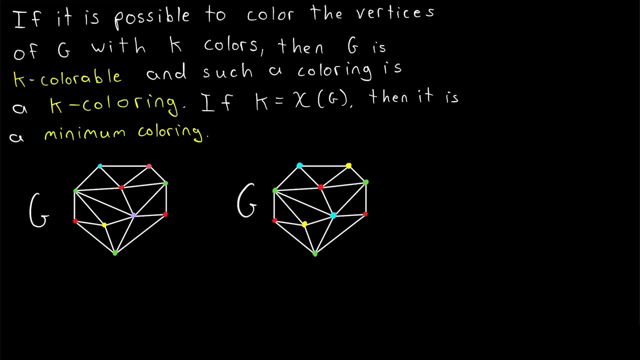 k is said to be k chromatic. All right, let's get down to our last set of definitions. If it is possible to color the vertices of a graph g with k colors, then g is said to be k colorable, and such a coloring, that is, a coloring of g that uses k colors, is predictably called a k coloring. 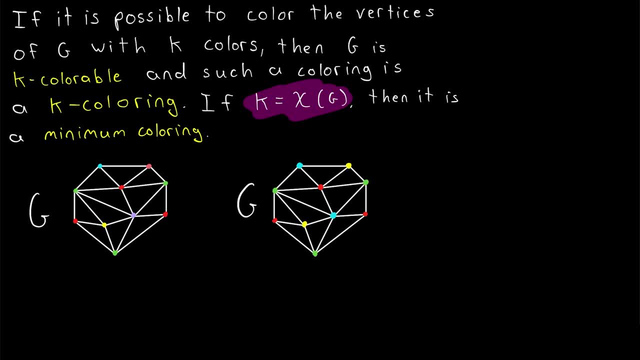 Furthermore, if k is equal to the chromatic number of g, then it's called a minimum coloring, because of course, it is a coloring of a graph that uses the minimum number of possible colors. Here we've got the same two graphs and the same two colorings that we looked at just a moment ago. Remember that. 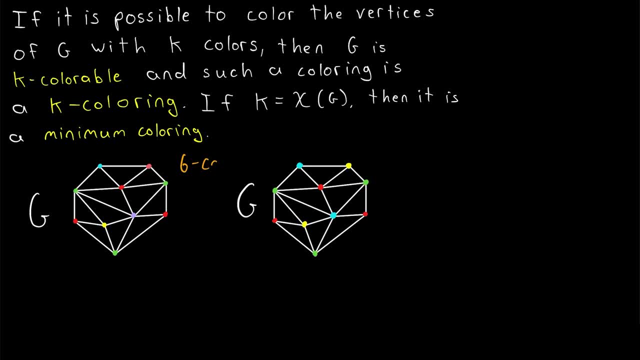 this first coloring used six colors, so this would be called a six coloring of the graph, And recall that the chromatic number of the graph turned out to be four. That's the minimum number of colors needed to color the graph. Thus, this six coloring is not a minimum coloring. We're using more colors. 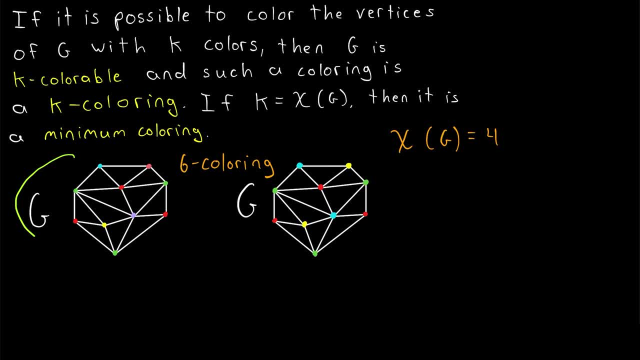 than is absolutely necessary. And of course, since we were able to color the graph with six colors, we could say that g is six colorable And in fact our graph g is k colorable for all integers k that are at least four, since of course that's the minimum number of colors necessary And k is bounded above. 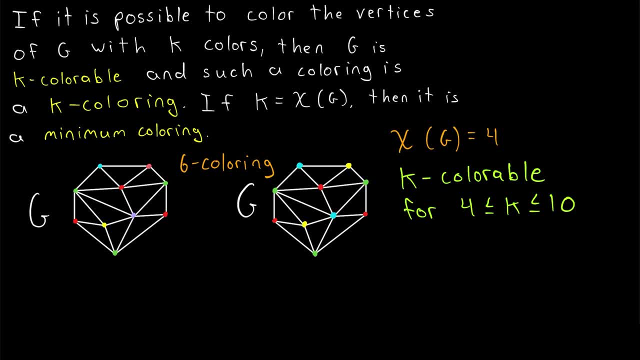 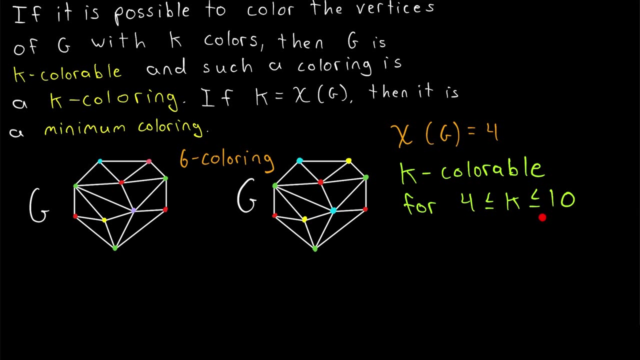 the number of vertices in the graph, which in this case is 10.. Certainly, if a graph has n vertices, we can't color it with more than n colors, because there wouldn't be enough vertices for all of the colors. So since our graph has 10 vertices, in this case we could color it with at most 10 colors. 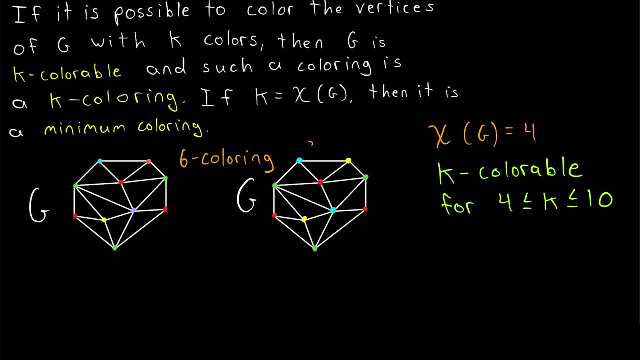 And remember that this coloring of the graph on the right was a coloring that used only four colors, which is the minimum number possible for this graph. You could call this a four coloring or a minimum coloring of the graph, And remember that this four coloring of the graph is called a minimum coloring because in this case, the chromatic number of the 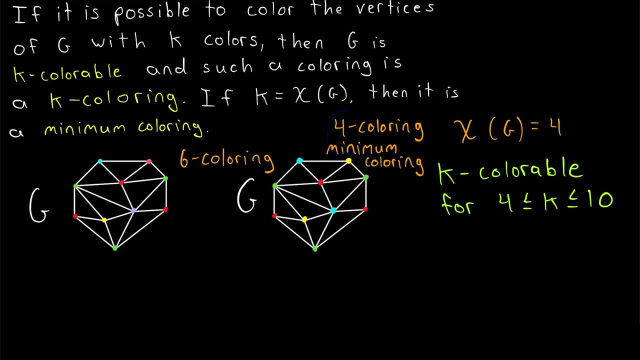 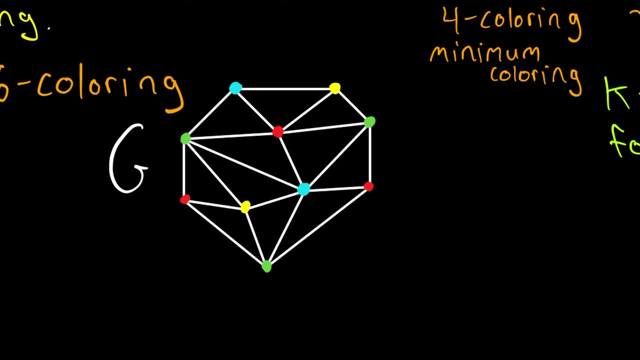 graph is equal to four. Alright, now let me shrink all of this stuff just to get it a little out of the way, and let's mention one more important thing before we go. As you can imagine, picking an arbitrarily large number of colors for different graphs is a bit of a hassle, So 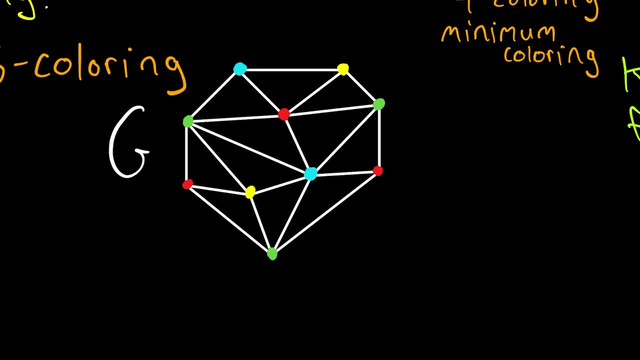 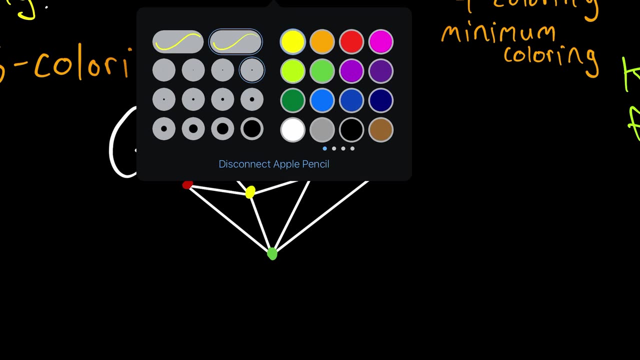 instead of actually using the names of colors, in practice we usually just use positive integers. So instead of assigning these two vertices the color blue, we might just assign them both the number one. Then we might assign the yellow vertices the number two. We might assign the 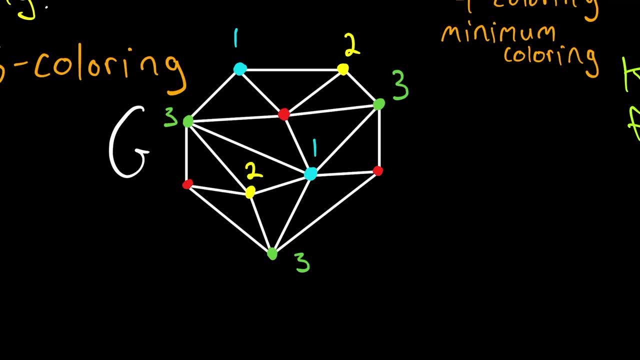 green vertices the number three, And then we might assign the red vertices the number four. So we can think more abstractly about colorings of graphs Instead of just thinking about them as an assignment from the set of colors to the vertex set of a graph. 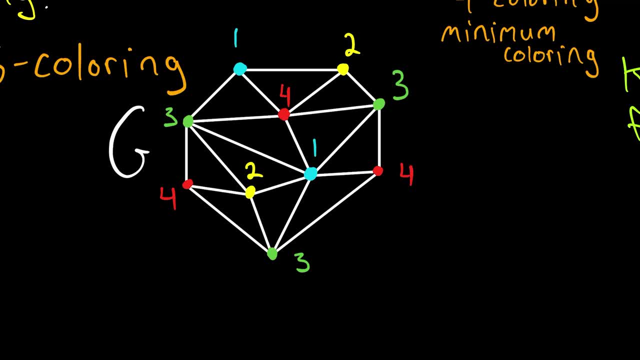 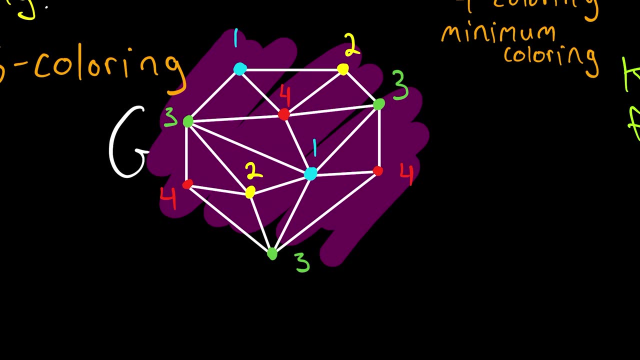 such that adjacent vertices are assigned different colors. we can think of a coloring of a graph as being an assignment from the elements of some set you can think of as a set of labels to the vertex set. In this case, we've assigned positive integers as our labels to the vertex. 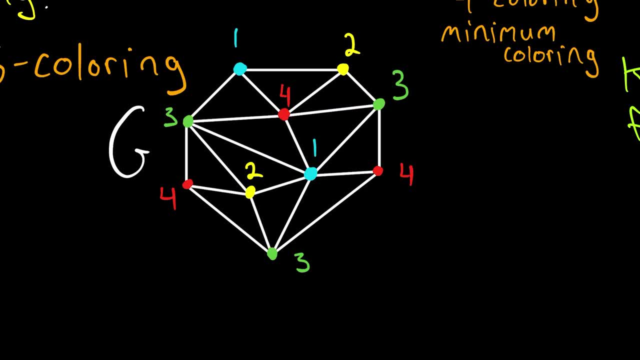 set of the graph and it's a coloring, because adjacent vertices have been assigned at different labels. This vertex labeled 4,, for example, is not adjacent to any other vertices labeled 4.. Thinking about graph colorings in this way makes it a much easier concept to work with in general. 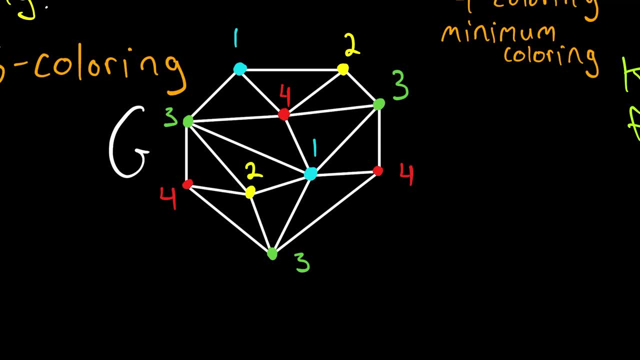 And talking about assigning labels to a set of vertices might make you start to think about functions. We'll talk about colorings as functions in a future lesson, but I encourage you to think more about the topic and let me know what you think down in the comments. So with that said, 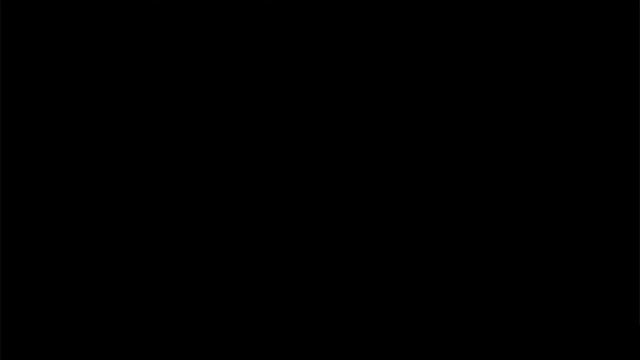 let's just take a look at one more small example for the road. Suppose we wanted to color the vertices of this 5-cycle C5. We might start at this vertex and decide that we'll color it or label it as 1.. Then this vertex can't be labeled 1, since it's adjacent to this vertex. but we could. 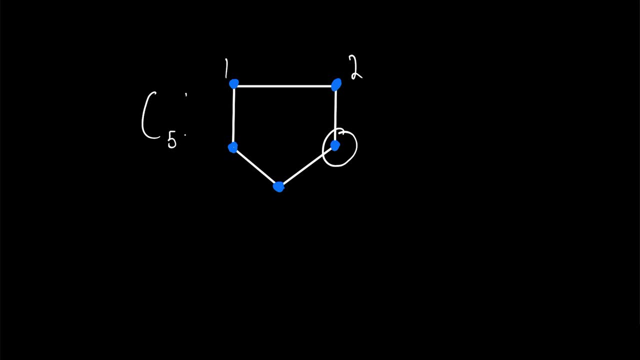 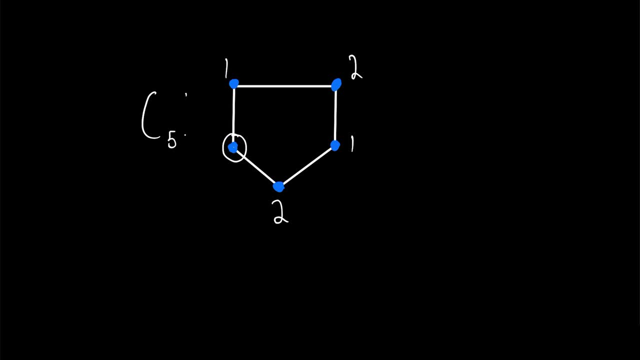 And then this vertex- here the last 1, is adjacent to a vertex colored 1 and a vertex colored 2.. And then this vertex- here the last 1, is adjacent to a vertex colored 1 and a vertex colored 2.. 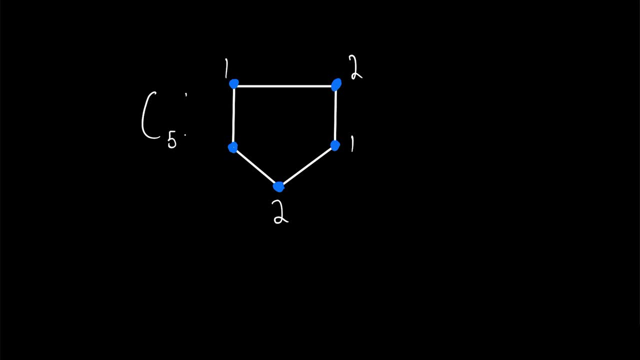 So here, with the last vertex, we've got to bring in a third color. so we'll color it three. And note that when I say we're labeling these vertices with a color or with a number, this is different from what we traditionally think of as a vertex labeling. 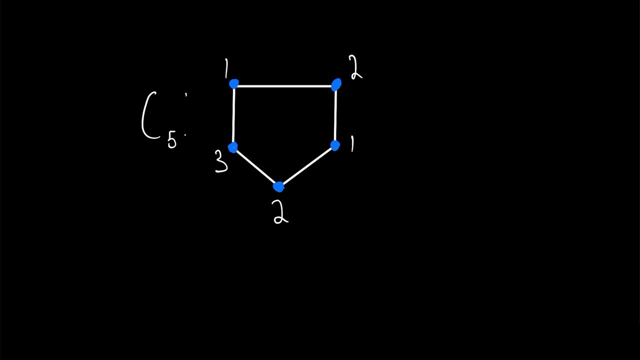 where each vertex needs its own unique label. And of course, And, of course, And of course, If you wanted to, just for fun, after coloring a graph like this with positive integers, you could assign a particular color to each positive integer you used. 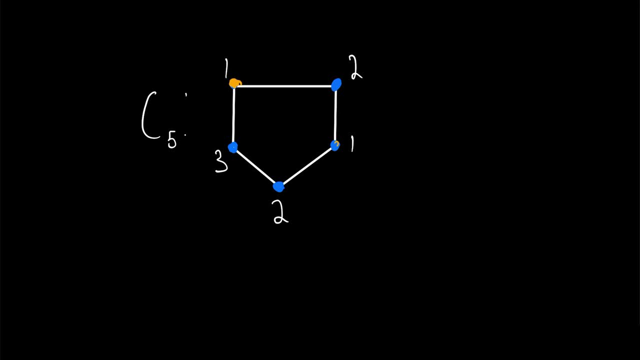 We could say the vertices colored 1 will be orange, the vertices colored 2 maybe will make those green, and then the vertex labeled 3 will be this sort of pink-purple color. One last time let's emphasize the definition of a coloring.